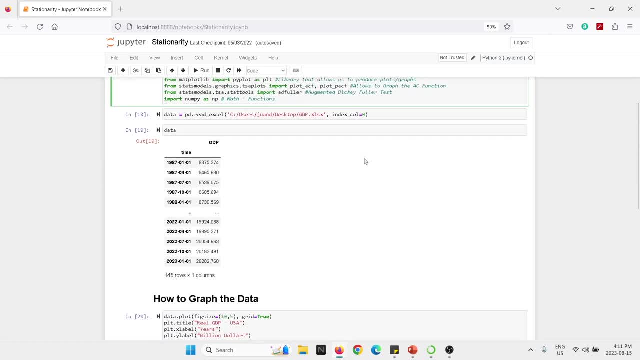 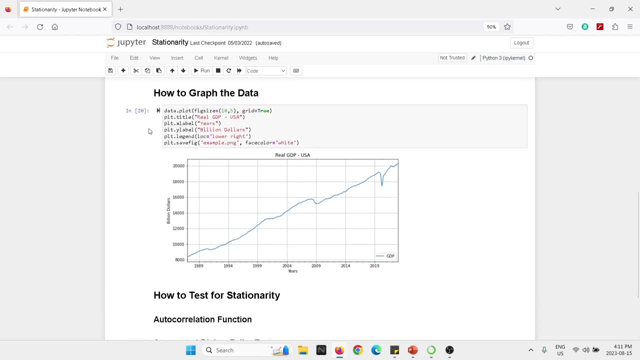 But so far we've learned how to import some libraries. Here we have the data set and here we have the graph. So the first step for the stationarity analysis is looking at the graph and seeing if the variable, for example, has a trend or has any sort of pattern. 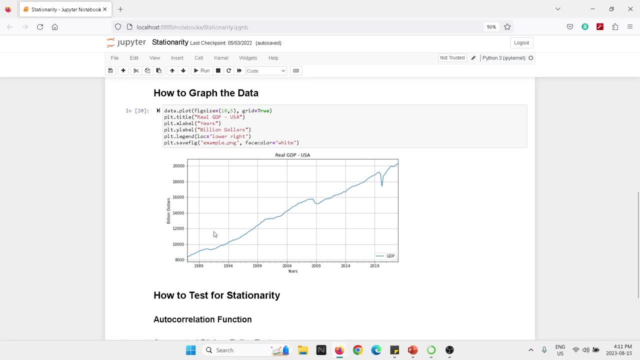 That is not a constant pattern. Normally on a stationary time series, you're going to see something that wiggles consistently around the mean. In this case, we don't see a series that is moving in a constant fashion around the mean. We're seeing that the series clearly has an upward trend. 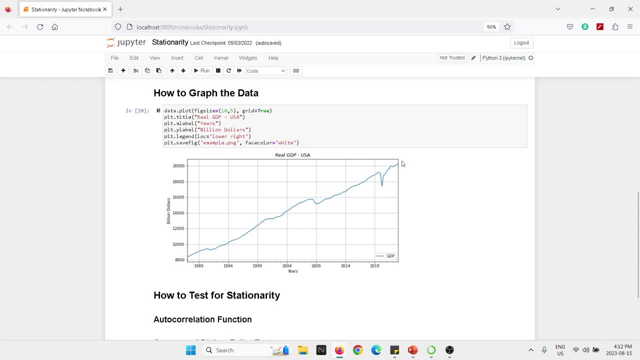 And this is already indicating us that the series is moving, And this is already indicating us that the series is non-stationary. However, if we want to deepen our analysis and try to determine whether the series is stationary or not, we will have to complement this with the autocorrelation function. 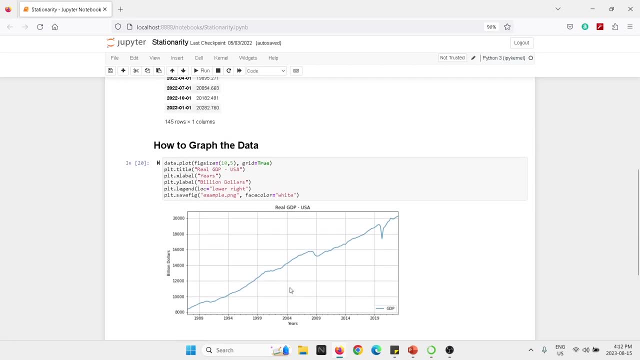 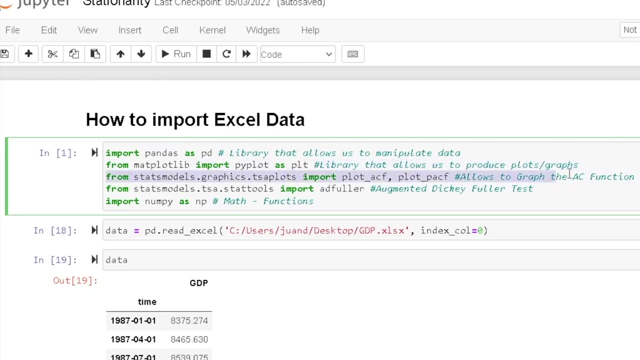 In order to produce the autocorrelation graph, we will need to import a library, And the library that we are going to be importing is the following: We're going to be importing the plot autocorrelation graph, Plot autocorrelation function and plot partial autocorrelation function from statmodels graphic to TSA plots. 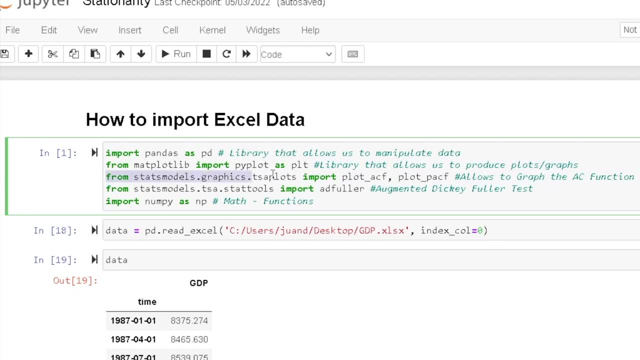 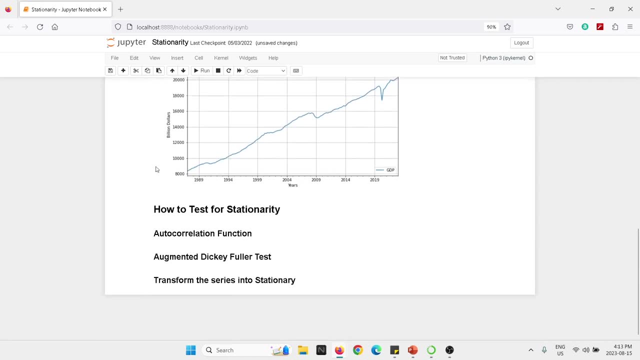 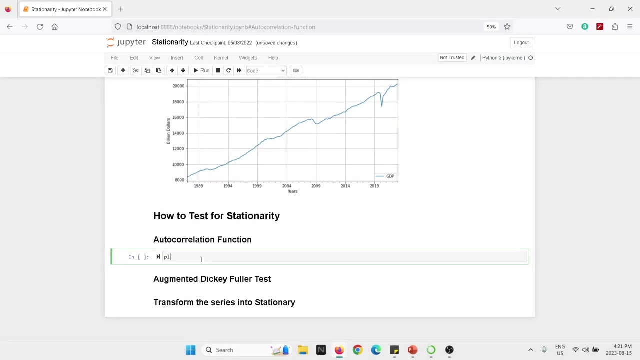 So you need to basically write this line And you're going to hit on run, of course, And now we will be able to write the code for the autocorrelation function To plot the autocorrelation function. we're going to type: plot underscore ACF. 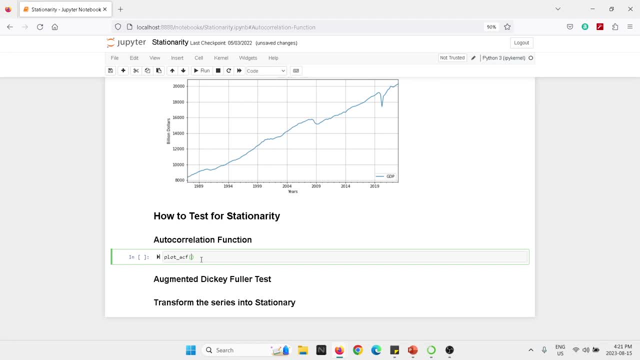 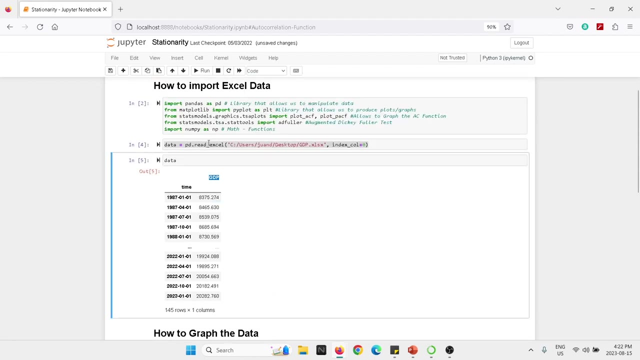 We open parentheses And now we have to specify what's the variable that we want to conduct the autocorrelation function. In this case, the name of my variable is GDP, And GDP is located in my data set that we have called data. 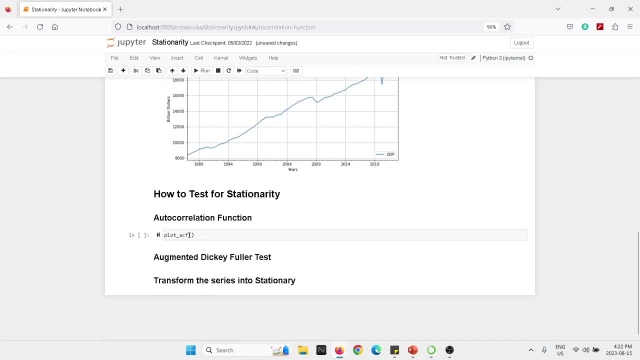 So I'm going to scroll down. I'm going here to specify the name of my data set. It is data And in square brackets I want to clarify that the name of my variable inside my data set called data is GDP. Next, I would like to include an option to determine how many lags I would like to include in the autocorrelation function. 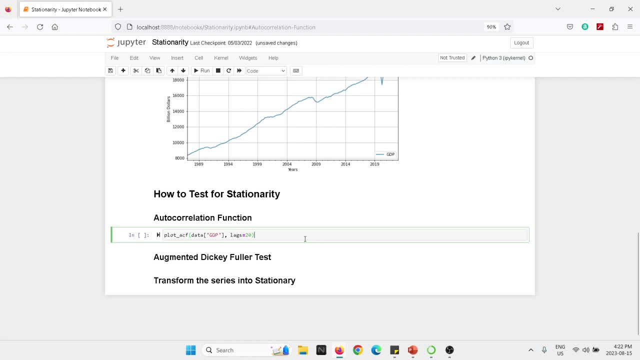 In this case, I would like to include 20 lags. Next we need to type PLT, dot, PLT, And this line is basically going to produce the plot of the autocorrelation function. I'm going to hit on run. 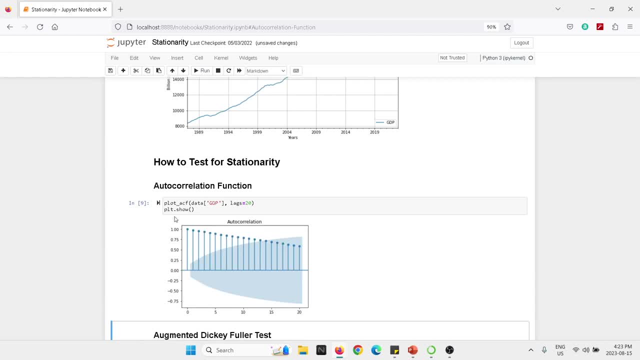 And here we get the graph. The way we're going to analyze this is the following: If the lags decay in a very slow pattern, which is the way that we can see here, it's indicating that our series is in a very slow pattern. 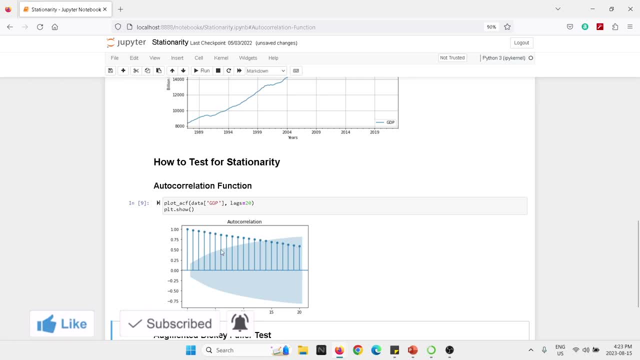 This is non-stationary. In a stationary series, the autocorrelation function is going to decay in a very fast pattern. You're going to see maybe a significant lag in the first spike or two, But then you're going to see that the lags will not be significant. 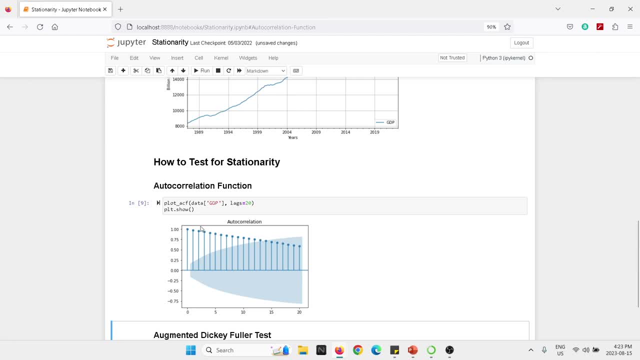 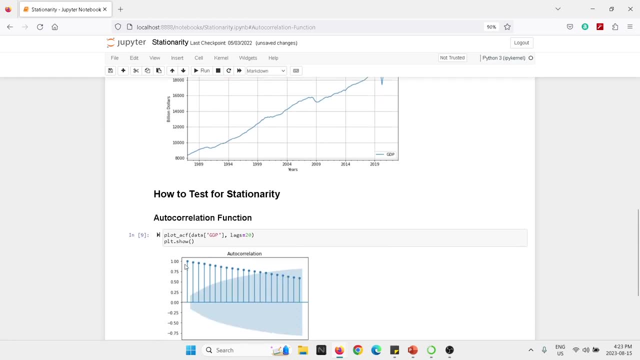 In this case, the autocorrelation function is suggesting that the series is non-stationary and that the series has a trend, which is what you can see in here. That's why the autocorrelation function is decaying in a very slow pattern. 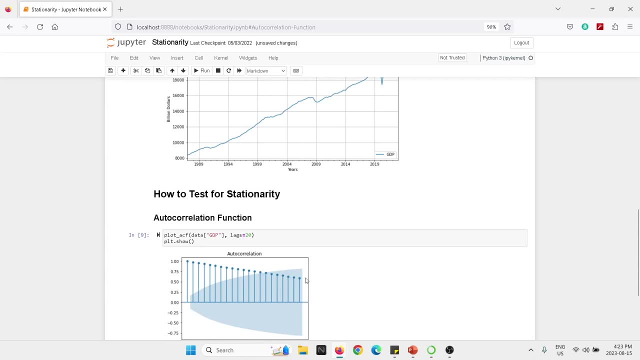 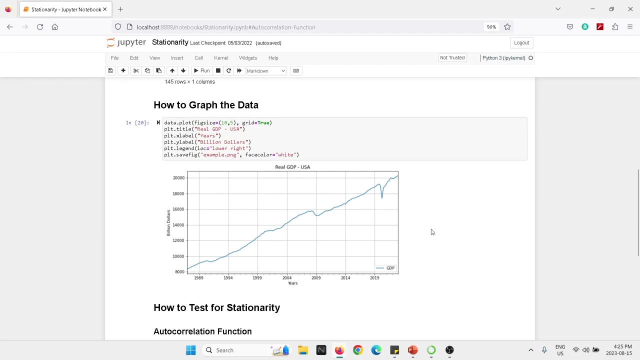 It's telling us that the series has a trend and is non-stationary. The final step is to conduct a formal test. So far, we have seen in the graph that the series has a positive trend, which is indicating non-stationarity. 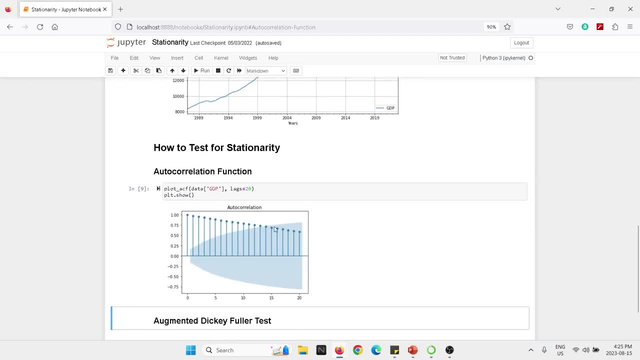 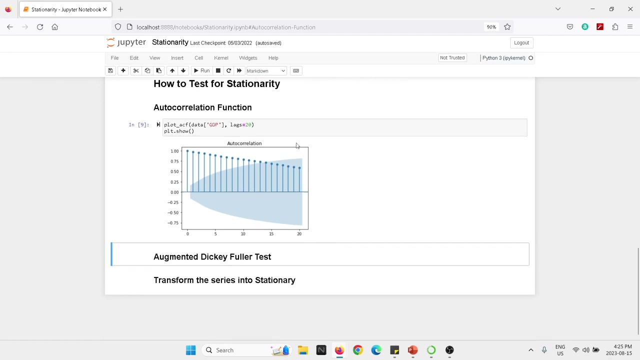 We have complemented the analysis with the autocorrelation function And we have determined that the lags decay in a very slow pattern, Indicating non-stationarity, And, furthermore, that the series has a trend. Finally, we're going to now conduct the augmented Dickey-Fuller test. 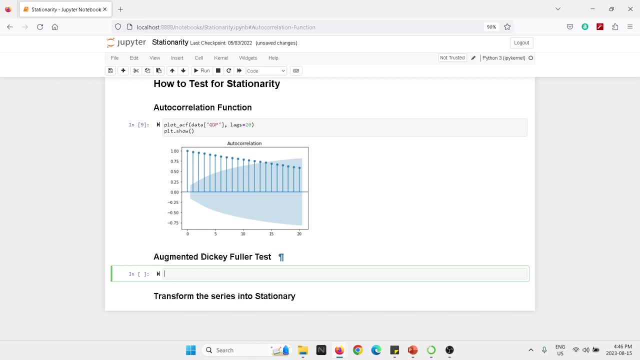 To conduct the augmented Dickey-Fuller test. first, we're going to specify where we would like to store the results. In this case, I would like to call it ADF test. Of course, you can assign the name that you wish. 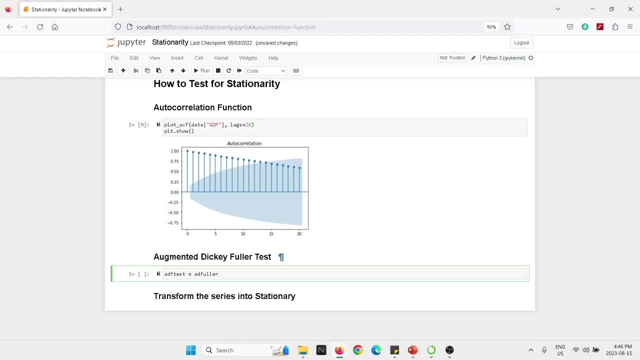 Then we're going to type ADFuller, We're going to open parentheses, And the syntax is very similar to the autocorrelation function. First, we need to specify the name of my variable. In this case it's GDP. 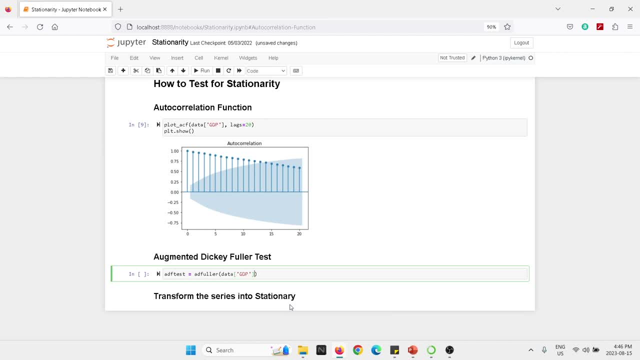 Sorry, Here we go Now. yes, Perfect. Then we need to specify how many lags we wish to include in the augmented Dickey-Fuller test. In this case, I'm going to use the auto-lag function. I'm going to let the software determine how many lags to include. 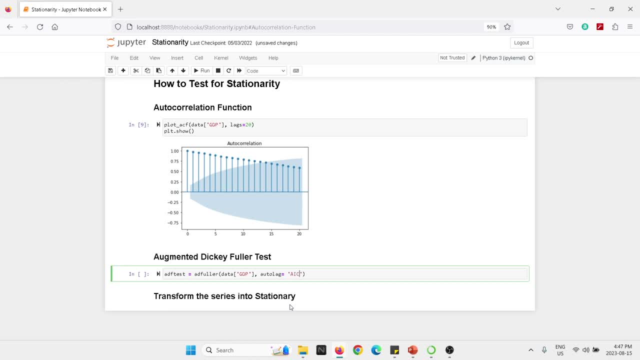 In this case, I'm going to use the Akaike criterion as the statistic to be used to determine how many lags to include in the regression. Finally, the last option that I would like to include in this case is going to be the option Regression. 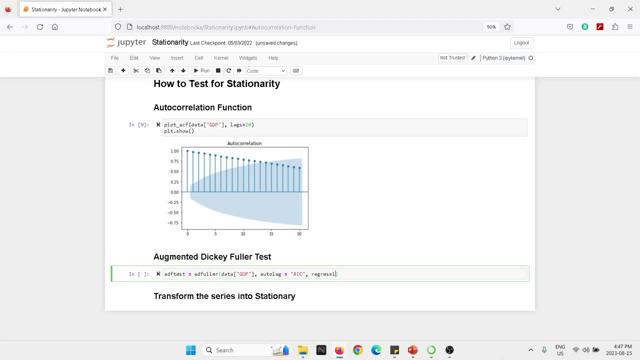 I'm going to type Regression And the option Regression is going to allow us to determine whether we would like to include a constant in the augmented Dickey-Fuller test. In that case, you're going to type C If you would like a constant and a trend. 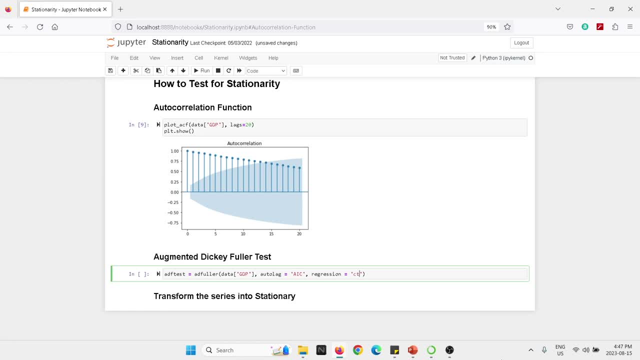 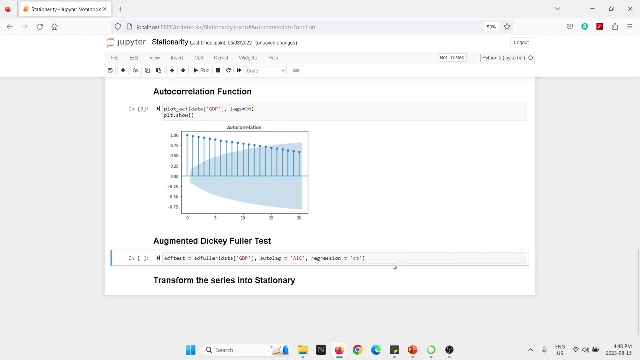 we're going to type CT, And if you wish no constant or trend, you would, of course, just type NC. In this case, we have determined that my series has a trend, so I'm going to type CT. I'm going to include a constant. 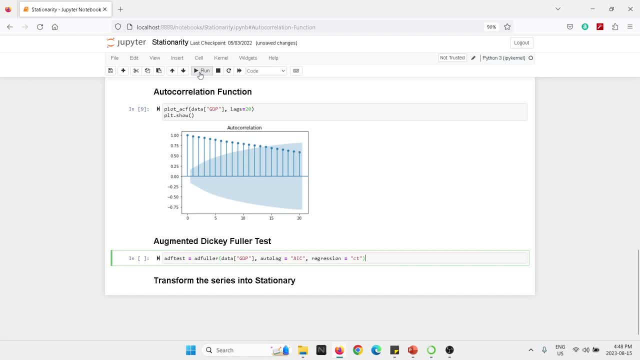 and a trend. So in this case, I'm going to hit Run now And you're going to see that we have not printed any results. We're not getting any results. All we did is basically run the augmented Dickey-Fuller. 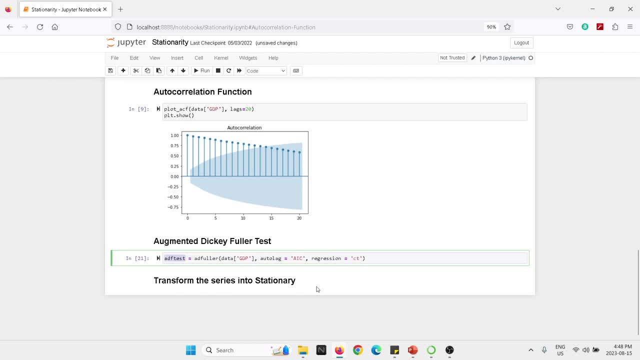 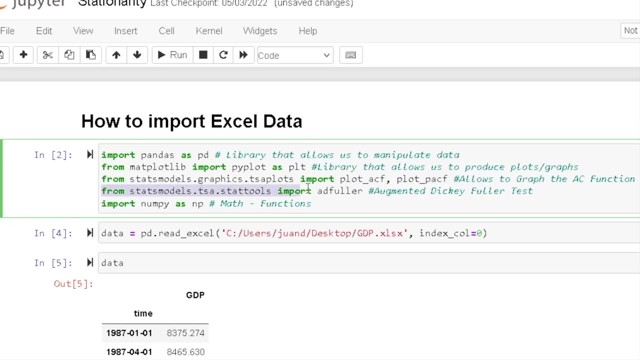 and store it in ADFTest. Also, another thing that I don't know if I mentioned, but I will mention it again just in case, is that we need to import the augmented Dickey-Fuller library. So you need to put from statsmodeltsastatTools: 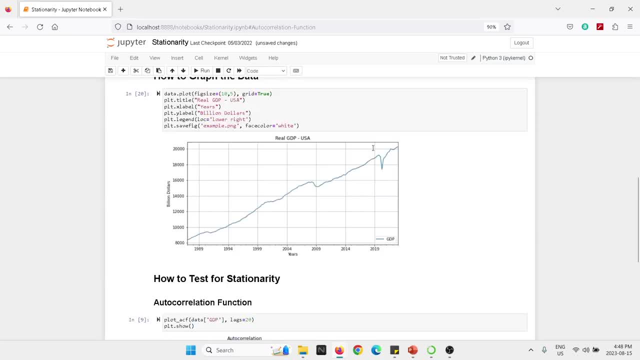 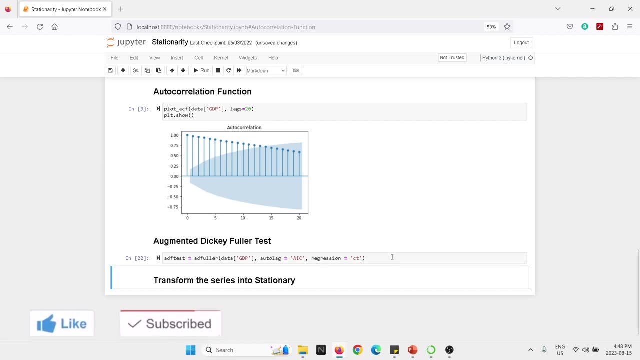 we need to import the augmented Dickey-Fuller. So if you don't do that, when you click on Run you're going to get an error saying: hey, I don't know what is ADFuller, I don't know this option. 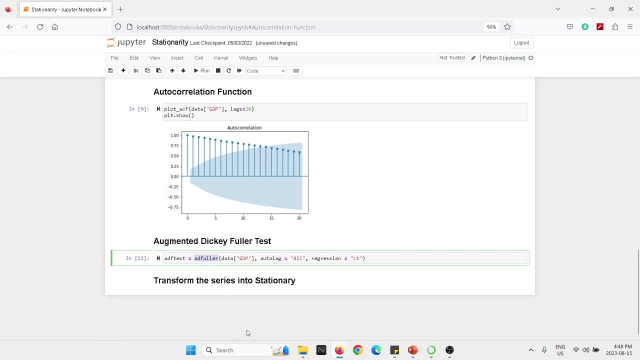 I don't know this command because you haven't imported that library. So anyhow, now to print the results. what we will need to understand about the augmented Dickey-Fuller is that it's going to be producing four results, five results actually. 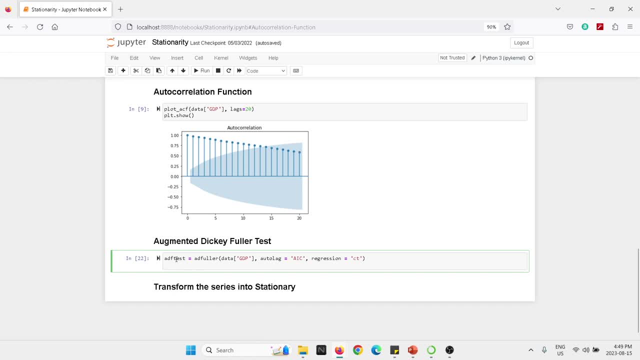 So these results are going to all be stored in ADFTest. So the values that it's going to be producing are five, like I just said, And in the first case, what it's going to be producing is the augmented Dickey-Fuller statistic. 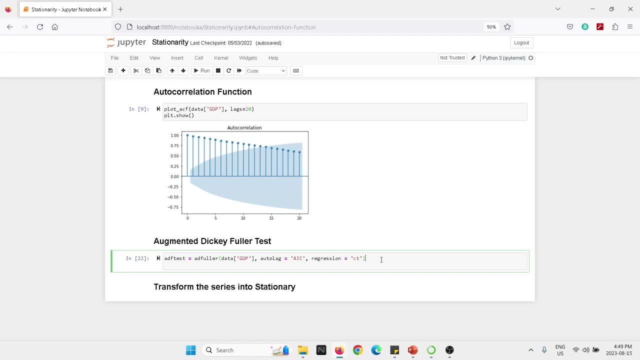 and that is going to be assigned the value of zero. So, in order to print that, we're going to type the following: print, of course, and we can print the. for example, we're going to type ADFTest, ADFTest. 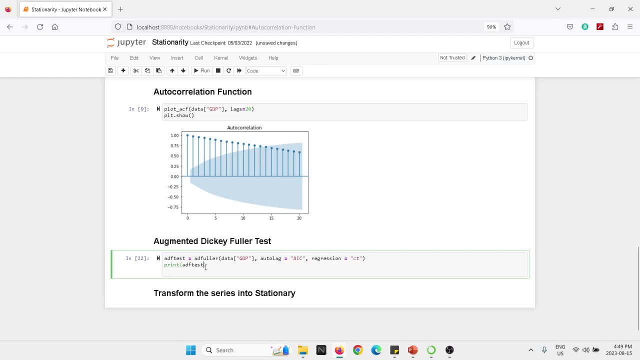 because the values are stored here in ADFTest. We open square brackets and we need the first value, which in this case is going to be zero, And we're going to see that it's going to print the value zero, which is the augmented Dickey-Fuller statistic. 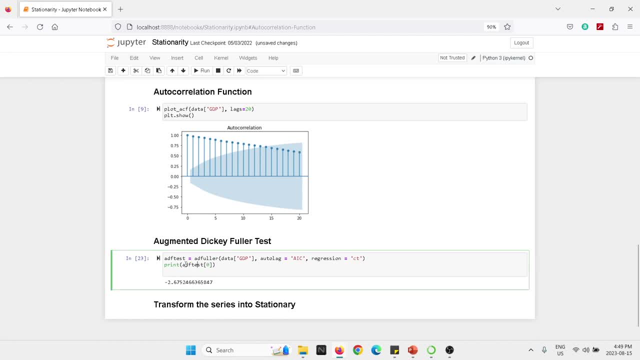 Now, if you wish this to say, ADFTstatistic, for example, we can print the name quotation marks ADFTstatistic, which is right, whatever you would like to write, of course, And there we go. We now hit on run. 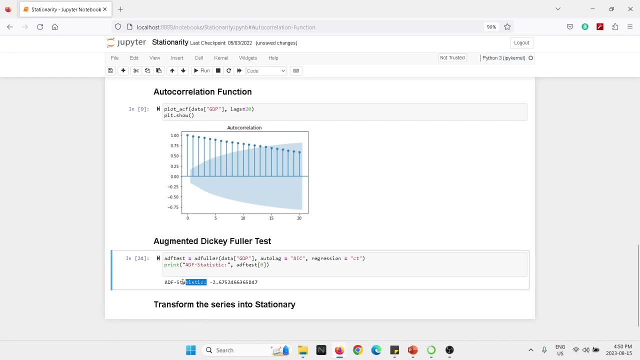 and you can see that we have produced the following. We have included the text ADFTstatistic. Now let's add a title print that's out: augmented Dickey-Fuller ADFTest results. Now we hit run. 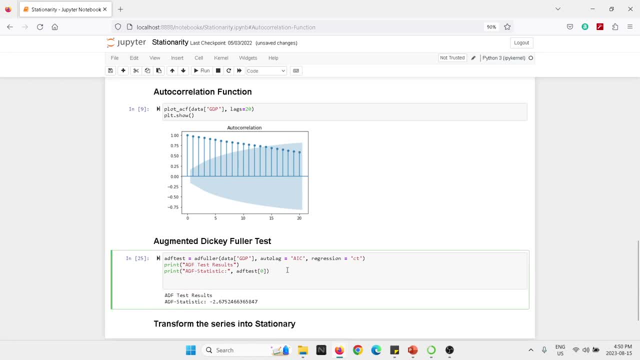 Now we get the title: ADFTest results. Now let's print another value stored in ADFTest. So the value, the first value that is going to produce, is the p-values. So let's assign a title here. 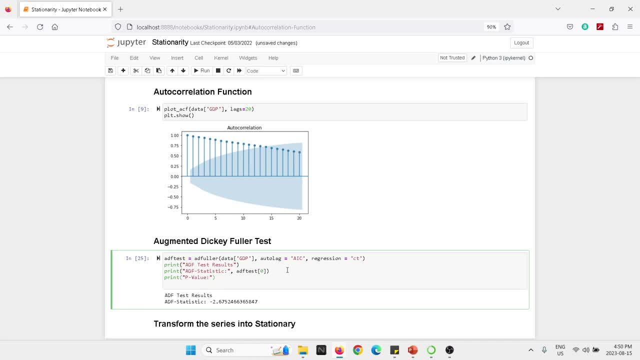 p-value- Semicolon comma. The first value stored in the ADFTest is the p-value. Now if we run, you see you get the p-value. The next thing that we can print is how many lags we have used. 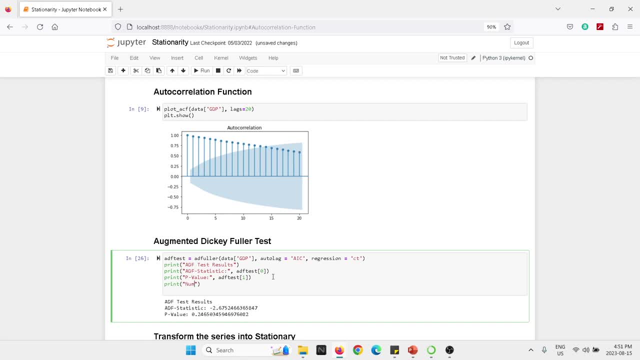 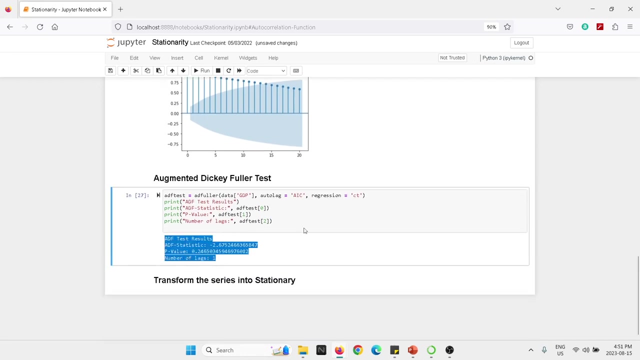 So let's add that Print number of lags comma, And we are going to include then the value stored. number two: We hit on run and here you get. the AkaiKey criterion has determined to include one lag in my augmented Dickey-Fuller ADFTest regression. 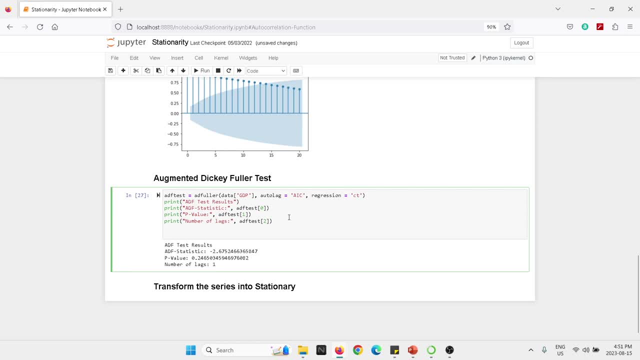 Now let's print the value number three. So print the value. number three is the number of observations in my regression. number of observations, Semicolon, comma. Let's put here comma ADFTest, and in this case, 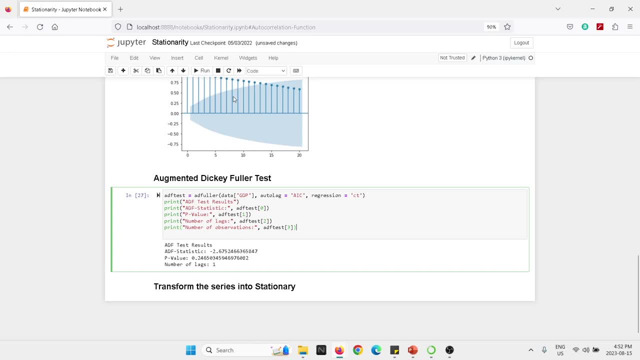 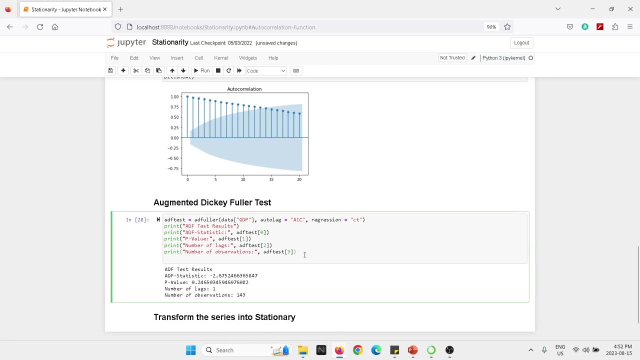 it's going to be the value number three. We can hit on run again and now you get here. we have 143 observations And finally, something we can print which is very important are the critical values. The critical values are stored. 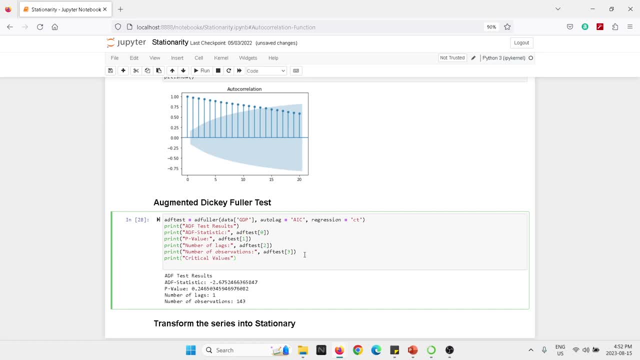 in the value number four. So critical values. sorry goes here ADFTest open square brackets. value number four: It's going to print all the critical values. You have critical value one percent, five percent and ten percent. 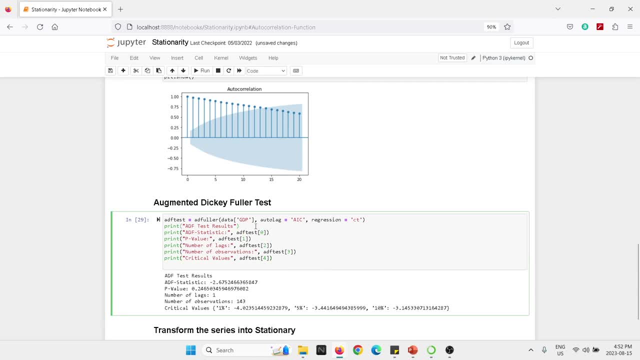 Something we can print as well, if you wish, is, let's print the null hypothesis. So we open quotation marks. null hypothesis. the series has and unit root. That's the null hypothesis. So here you see, we get the null hypothesis. 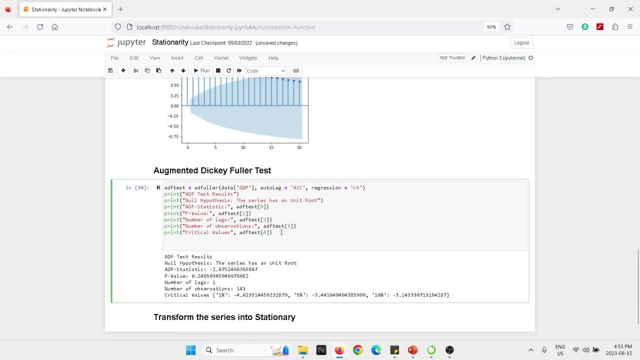 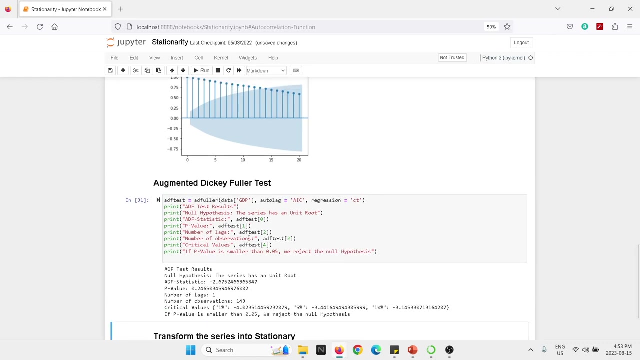 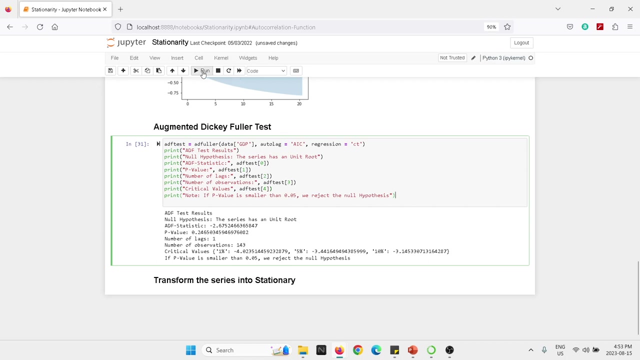 the series has a unit root. and the last thing that we can print, let's do the following, just as a reminder: if p value, we reject the null hypothesis, Let's put it as a note there. So now we have all. 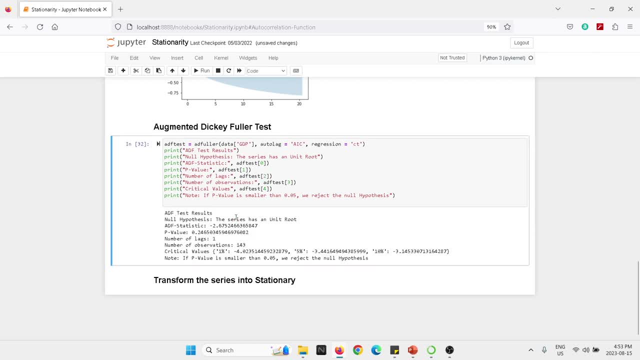 now the augmented DQFiller test results. It says the null hypothesis, the series has a unit root. we get the augmented DQFiller statistic, the p value, number of lags, number of observations, all the critical values. 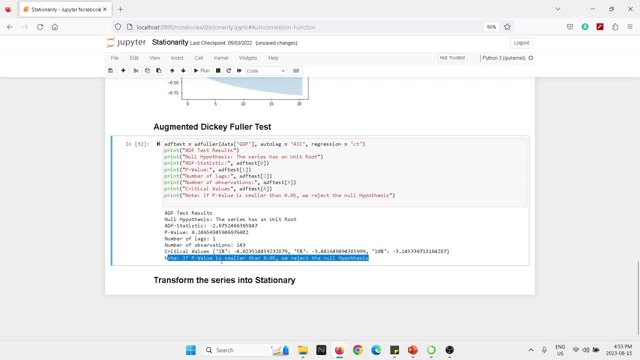 and we just wrote here a note, a reminder: if the p value is smaller than 0.05, we reject the null hypothesis. What is the null hypothesis? My series has a unit root. Now can we reject this hypothesis based on the p value? 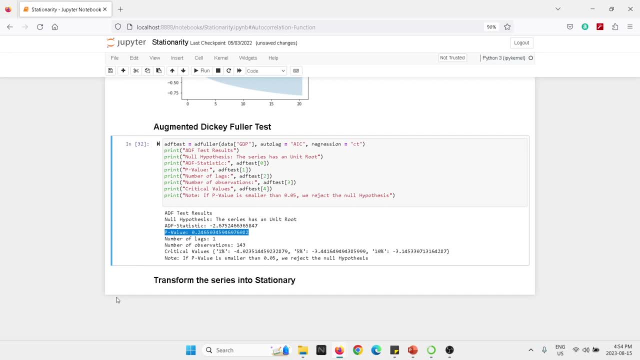 No, we cannot reject the null hypothesis because the value is bigger than 0.05.. Now, because the value is bigger than 0.05, we determine that my series has a unit root and therefore my series is non-stationary. 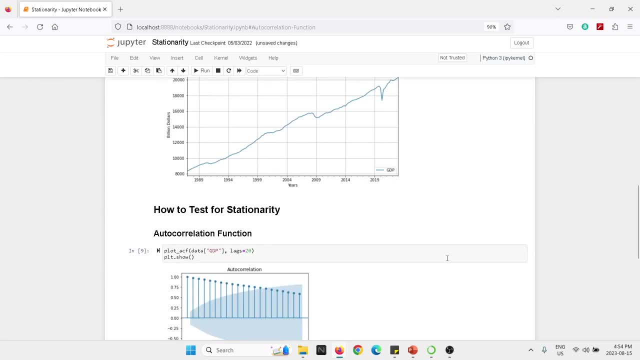 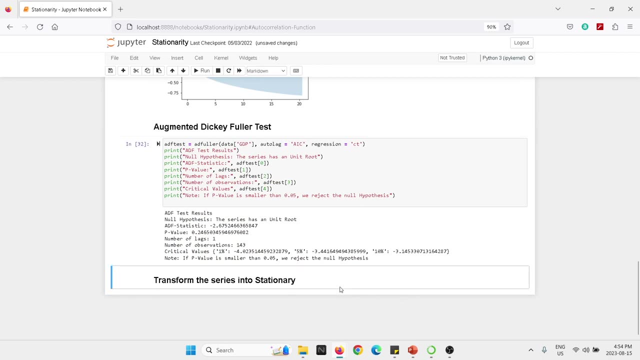 We have seen that the series has a positive trend and we have also complimented that with the autocorrelation. Now, how are we going to transform the series into stationary? Now, let's see how to transform the series into stationary. As you know, 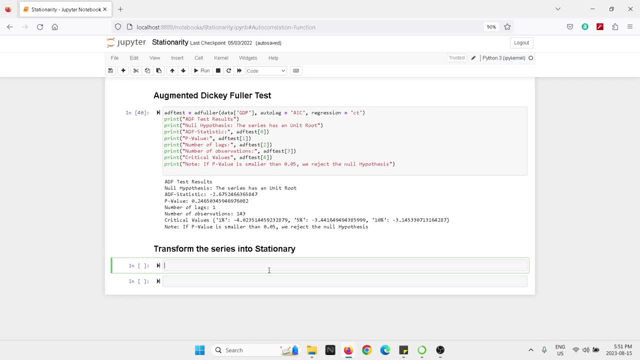 to try to estimate any sort of models, we need our series to be stationary, So, in this case, what we are going to do, then, is to apply a couple of transformations into our variable, So I'm going to write here a title. 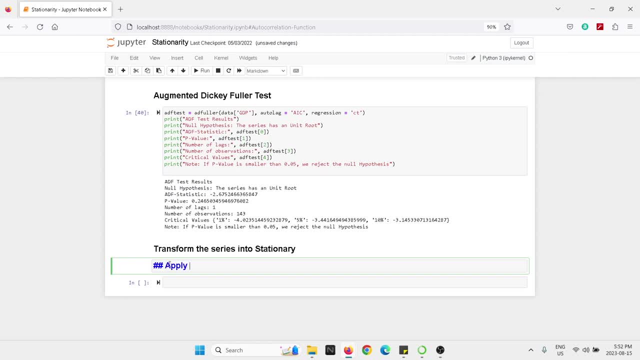 and we are going to be applying logarithms, differences, and then multiply times 100.. This is going to give us the series GDP growth, which is basically the percentage change, the quarterly percentage change. So I'm going to explain a little bit more. 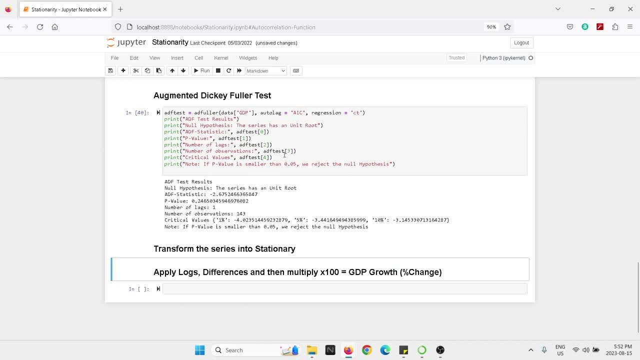 why we are doing this transformation. When the series is non-stationary and it has a positive trend, we need to detrend the series. We are going to be doing this applying differences. Now, when you apply differences, as I just mentioned, 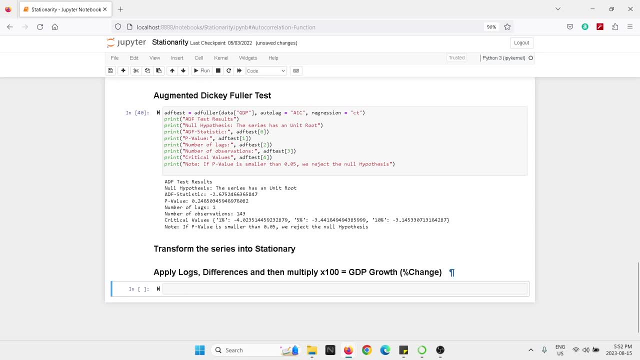 you are detrending your series and we are going to be applying logarithms and multiplying times 100. So any time we estimate a model, we will be able, first of all, to interpret the results as percentage change. That's going to be very helpful. 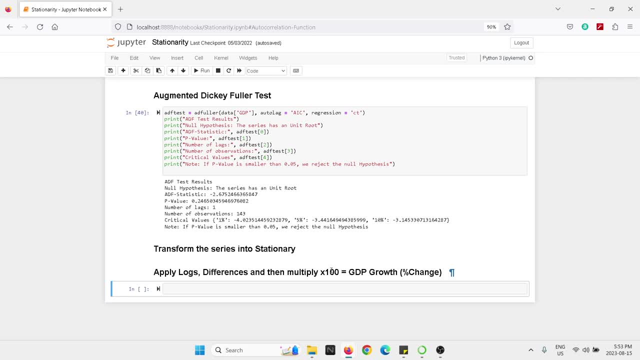 when we want to explain the results of any model And also, as I just mentioned, to be able to obtain the percentage change between each quarter of GDP. So, to start, we are going to be applying logarithms, So I'm just going to write here. 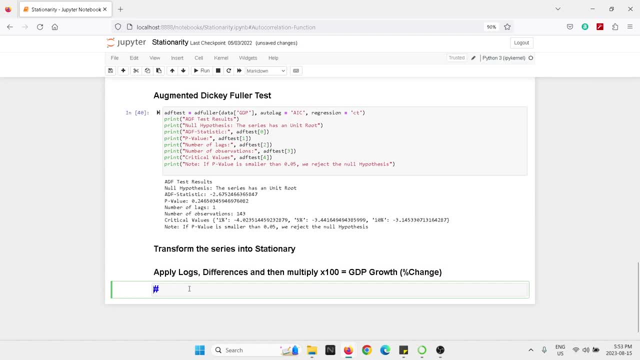 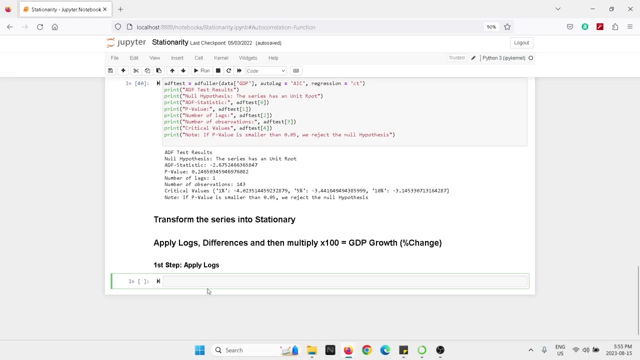 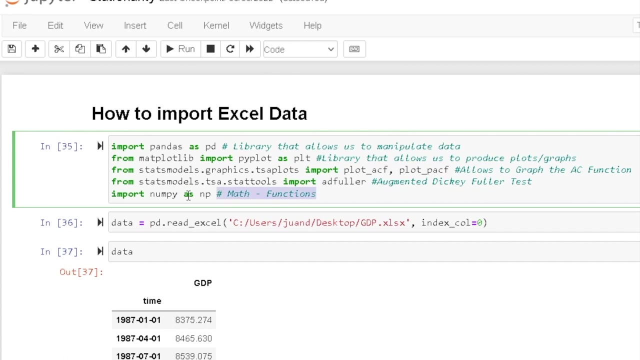 yeah, I'm just going to write here a subtitle and maybe let's go with. the first step, then, is apply logs. To apply logs, we need to first of all import the library numpy as np, So numpy is going to allow us to. 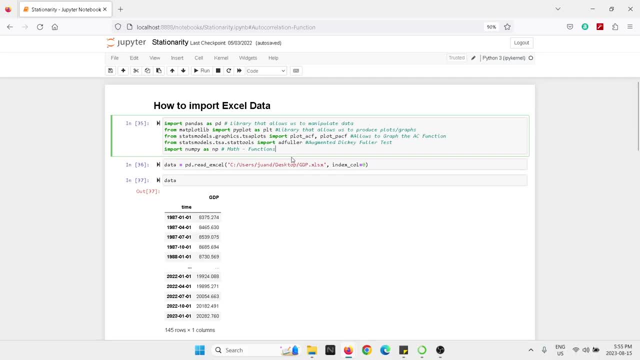 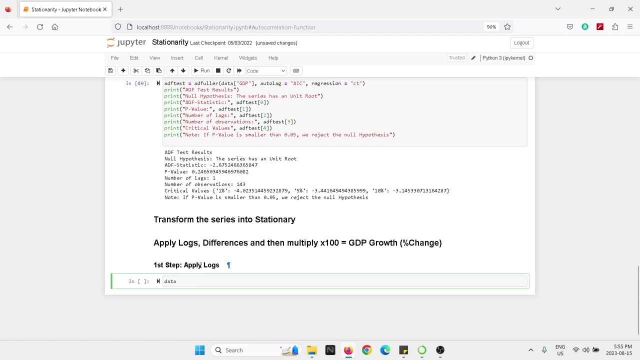 implement mathematical functions. In this case, we need to apply differences, logarithms, all of those transformations. we need to import that library And the first step is we're going to be creating a new variable, which we're going to call it. 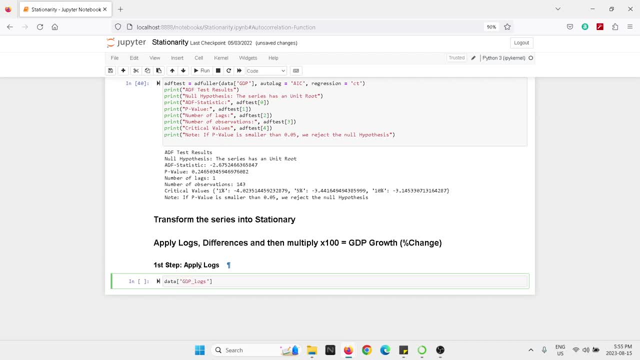 for example, gdp underscore logs And we need to next apply logarithms. So I'm going to type np, so we are using numpy log and then data. we have to determine on which variable we want to apply logarithms. 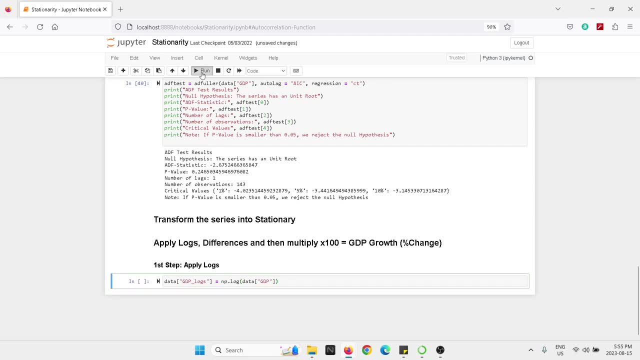 And it has to be on the variable gdp. We hit, run and perfect. Now we have generated my variable gdp logs. The second step is to apply first differences. So I'm going to create another title here. So 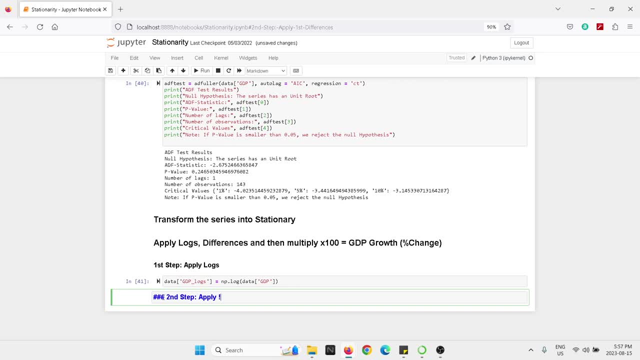 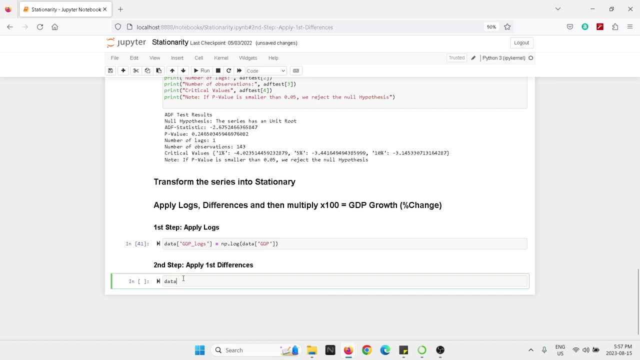 second step: apply first differences. To apply first differences. we're going to be doing something very similar. We're going to create a new variable, in this case gdp underscore div equal to now. we have to again determine on which variable we want to apply. 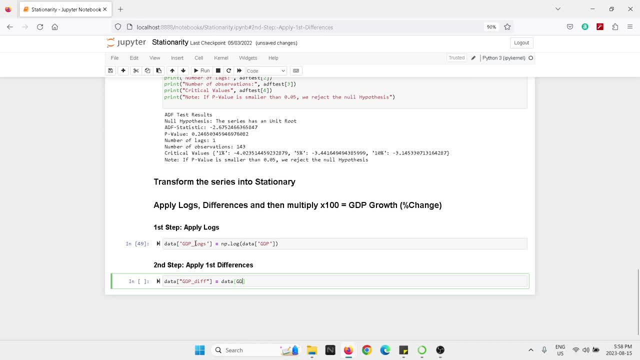 the first differences And we want to apply it on gdp underscore logs. All right, we need to apply first differences on my variable transforming logs And then you just type differences like this and parentheses. You hit on run. 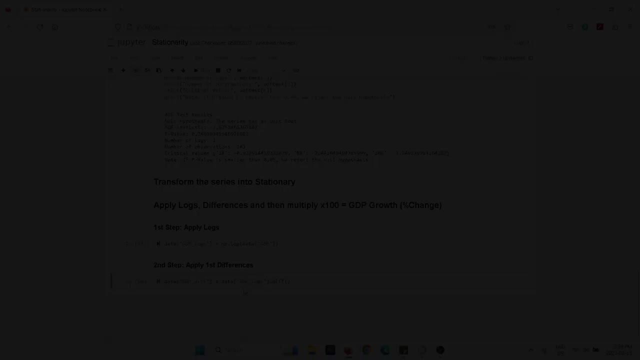 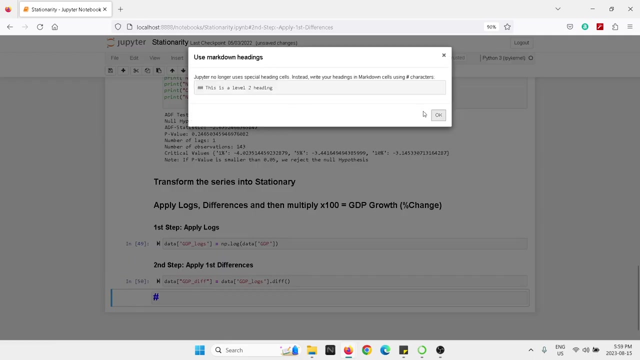 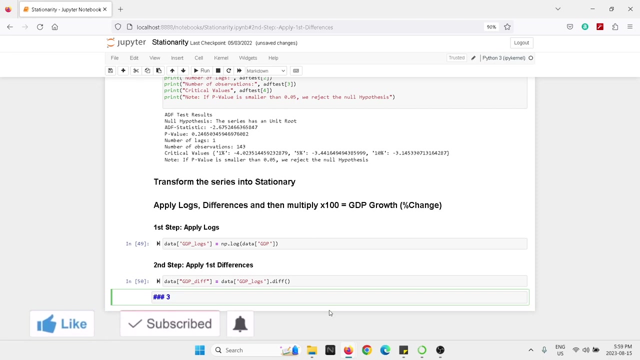 and now we have applied first differences to my series in logs. Now the third step is to multiply times 100, my series in logs and differences. So we're going to write third step. Sorry about that. Third step is multiply. 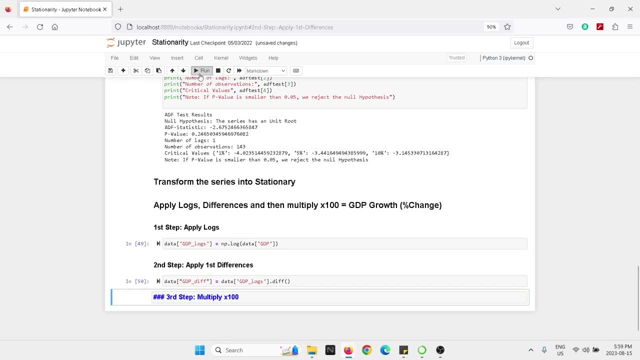 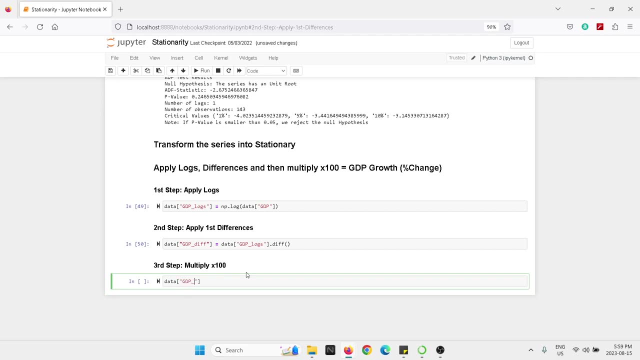 times 100.. So to multiply times 100, again, we need to create a new variable. I would like to call it gdp underscore growth. That's going to be the name of my variable And we're going to type the following data: 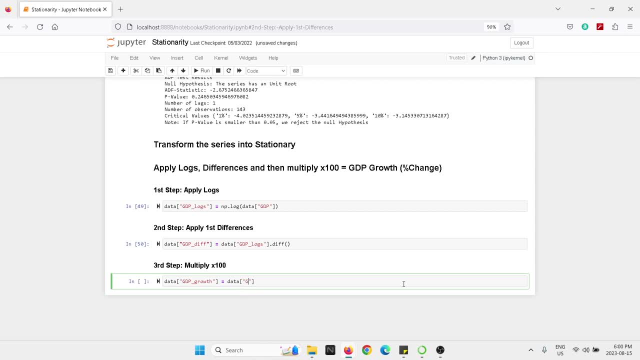 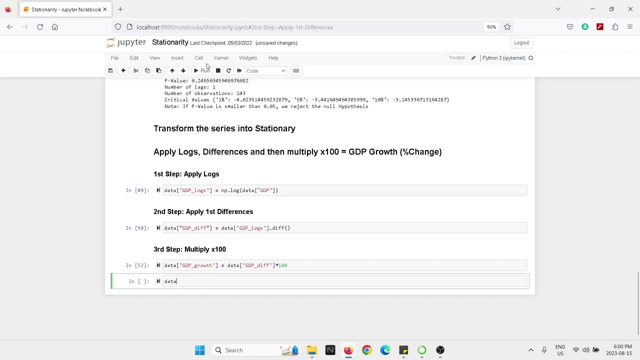 We need to call again my variable. In this case it's gdp in differences, And all we're going to do is multiply times 100.. We hit on run And here we go. Now I can type again data. Just hit on run. 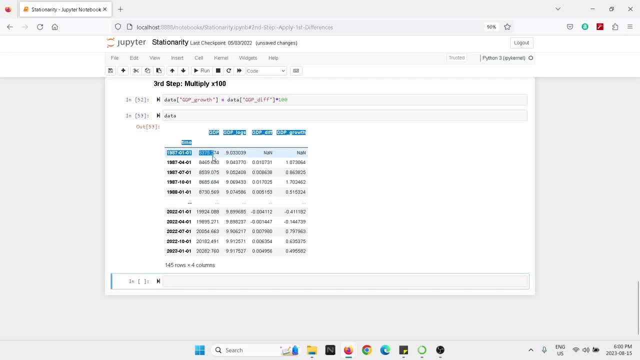 And now we can see, of course, that we have my series gdp. This was my original series. Then we have my series transform in logarithms, I have my series in differences And I have my series growth in growth. What we can do: 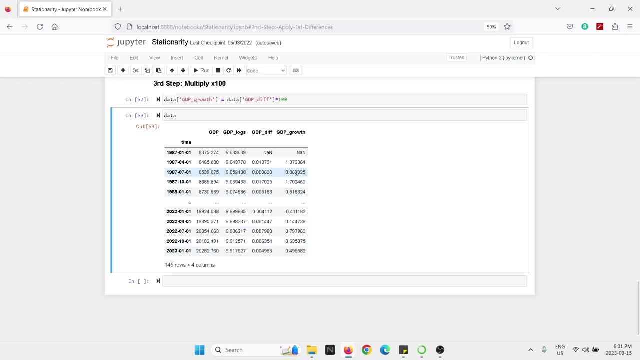 is, of course, graph the series. Something that I want to mention is: you're going to see, the first observation is missing because, in differences, you're subtracting the previous observation, The first observation, of course. then, for the first case, 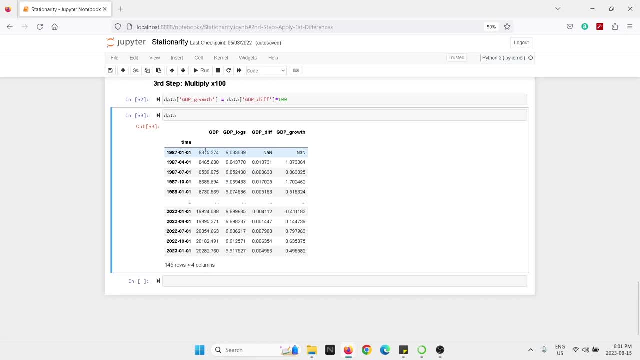 there's going to be no value because there's nothing before this observation. So that's why we cannot compute this value, But for, of course, all of the rest of the observations we do have a numerical value. Now we're going to produce. 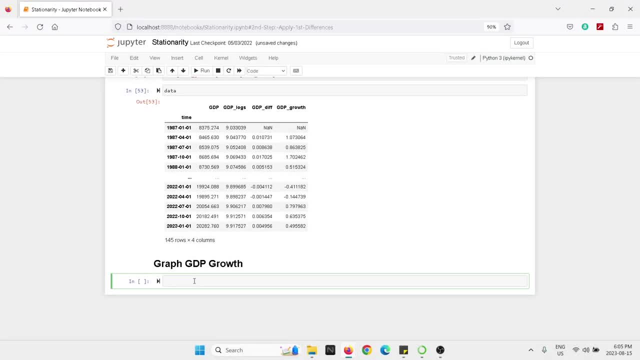 the graph and see if my gdp growth series looks stationary. We're going to type data, open the square brackets and we have called the series gdp underscore growth- Growth. There we go, And then we need to put dot plot. 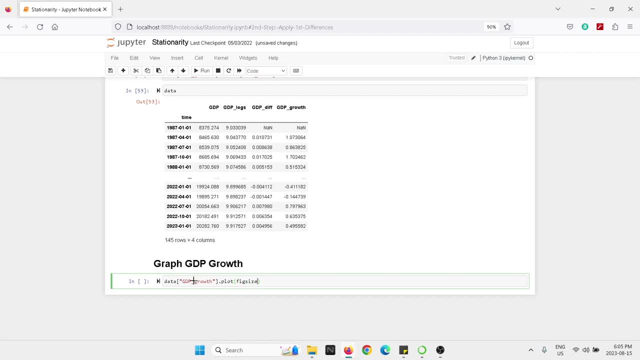 So some options. We want the figure size to be specific. We're going to put 10,, 5.. And we would like the grid to be in place. We can add the title PLT. title: gdp growth for USA. 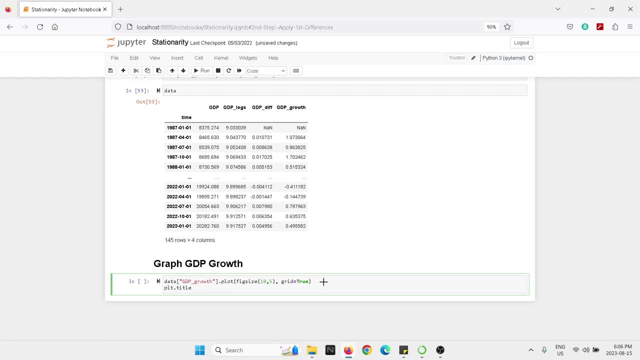 And then we can add the gdp growth for USA And then we can add the gdp growth product activity to the gdp growth platform. So we can add the gdp growth to the gdp growth platform And then we can add: 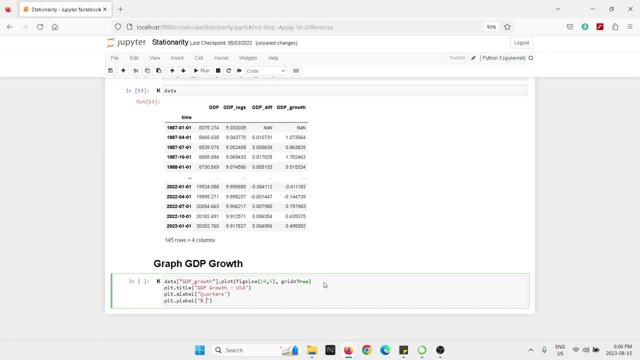 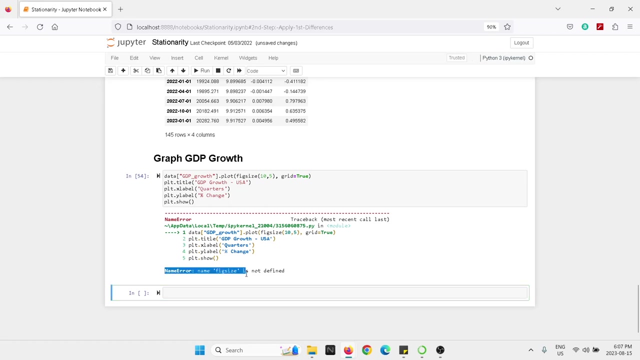 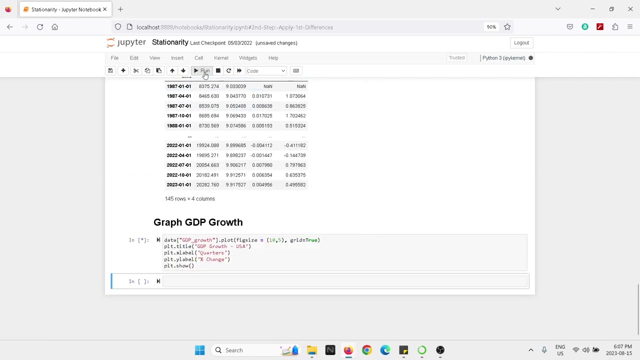 the gdp growth product to the gdp growth platform. So let's see now if we get the graph. we're getting an error. it says fixed size is not defined. we have to basically include an equal here. so now let's run again. and now, yes, here we go and we can see that we're getting the graph for GDP growth. 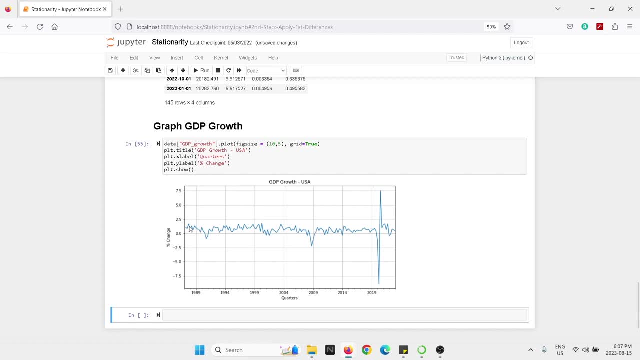 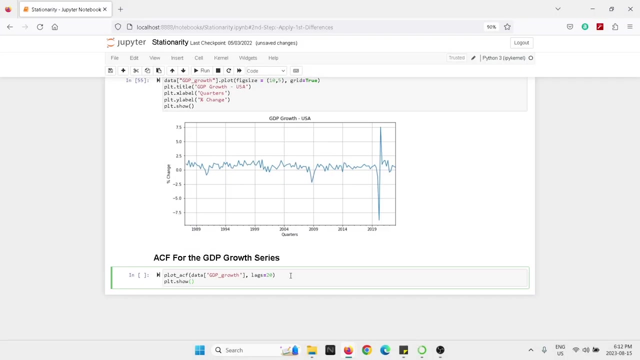 and this is how a stationary series should look like. as you can see, it's wiggling consistently around zero. of course, what we can see is there's a very significant peak here in during COVID. there's a big, big drop and a big peak in here, but overall, we can see that the series does look stationary. now let's 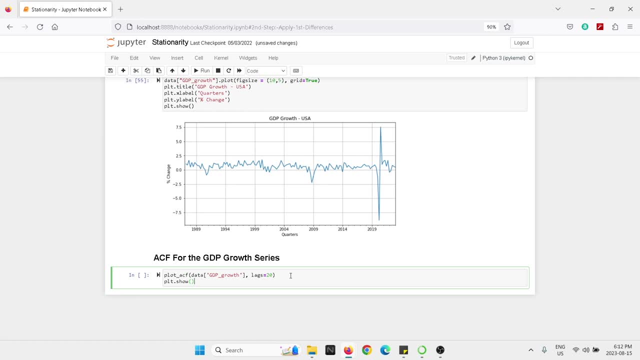 produce the autocorrelation function of my GDP growth series to see if the autocorrelation function looks stationary. we're gonna hit on run here. and we're going to run the autocorrelation function of my GDP growth series to see if the autocorrelation function looks stationary. we're gonna hit on run here. 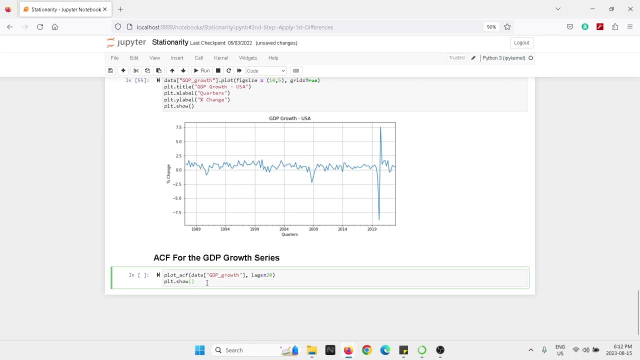 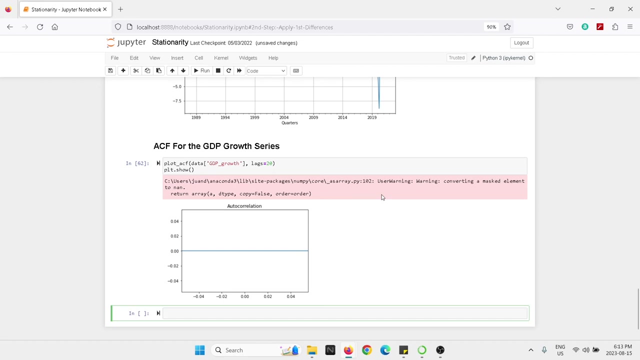 I just copy-pasted the same code than we did before. we already know how to generate the autocorrelation function. just make sure that you are putting here GDP growth. that's the name of the variable. I'm gonna hit on run and here we're getting an error. and that's great that we're getting this error, because I 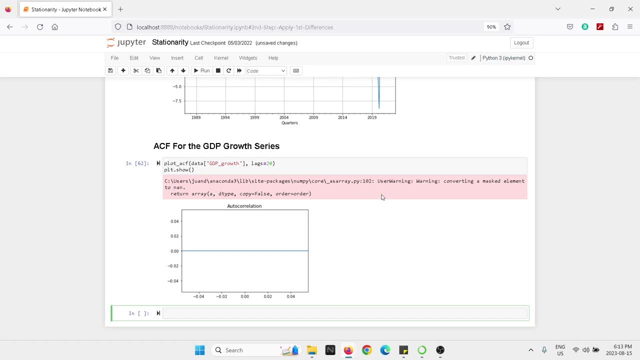 want to show you now how to fix this error that is going to be very common when you're working with a time series data. so we're getting a warning that says converting a masked element to a null. so basically, the error is suggesting that we have observations. 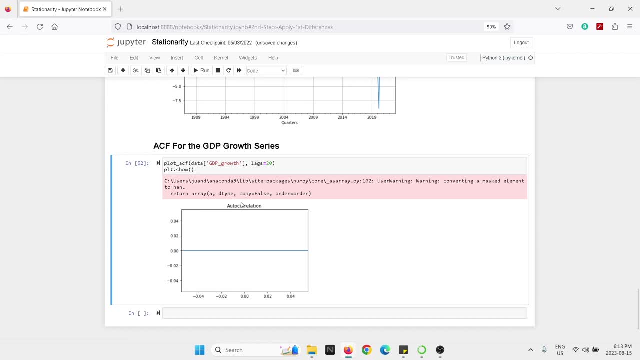 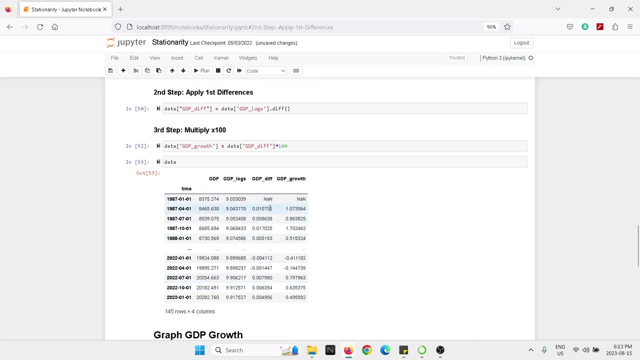 that are non-valid, that are empty, that are blank cells if we scroll up, remember, when we apply differences, we had subtracted the first observation and that's why here we're getting some cells that have no values, right? so the first column, the first cell- sorry, the first row- has no observations for GDP. 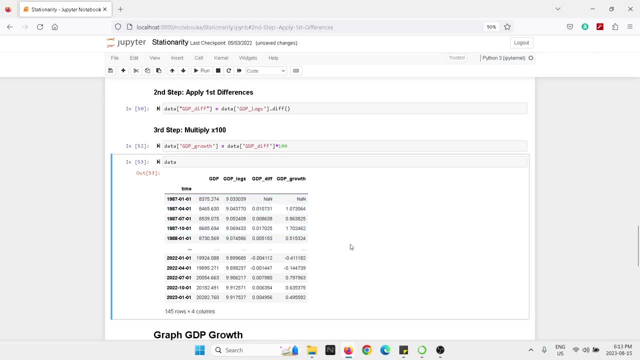 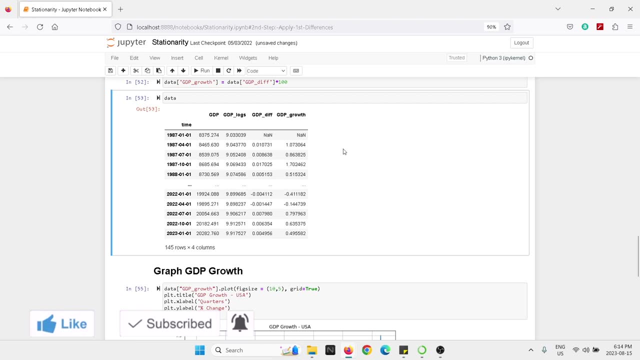 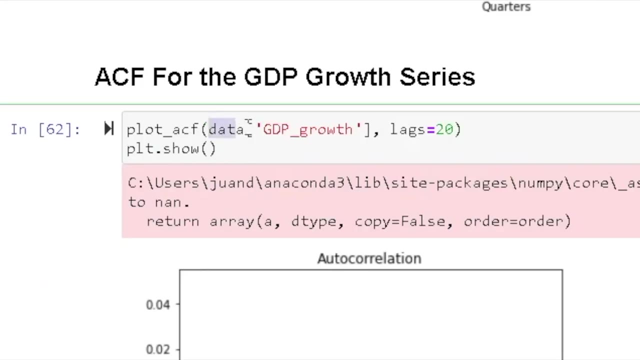 indifferences and GDP growth. So if we want to produce the autocorrelation function, we need to drop the first row. We need to drop the observations that are empty or non-valid. In order to do that, it's very easy. All we need to do is we're going to go into this portion of the code. 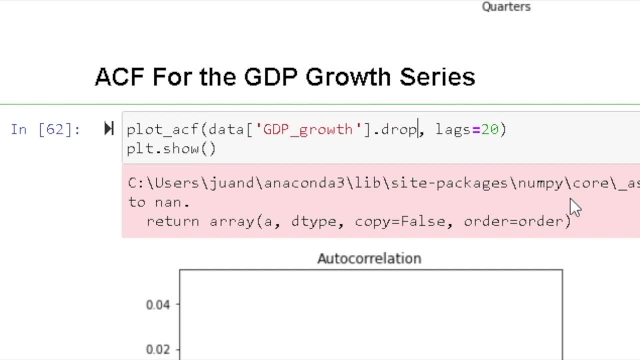 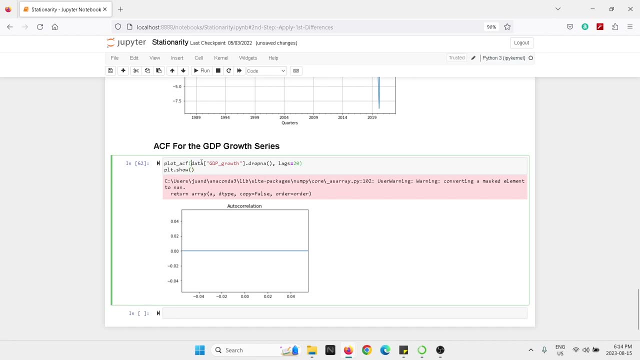 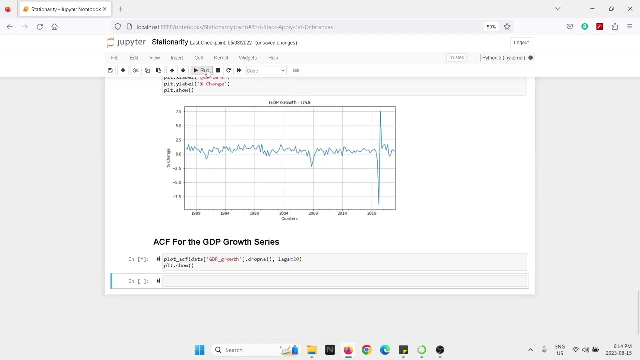 and we're going to type dropna open and close parentheses And basically we are saying here from this series, make sure you're dropping the non-valid observations or empty observations. Now I hit on run and here we get the autocorrelation function. 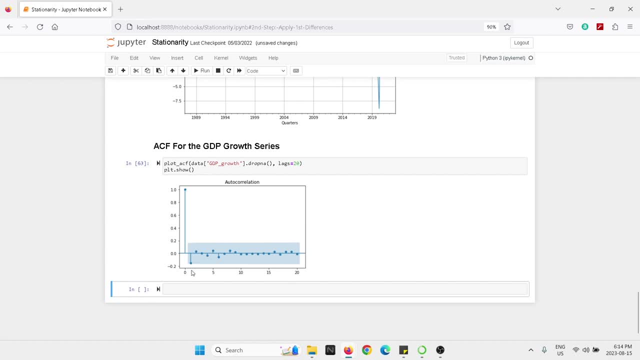 And now you can see that the decay is immediate. Remember before, when the series was non-stationary, the decay of the autocorrelation was really slow. I'm going to scroll up and I'm going to show you that the decay is really slow. 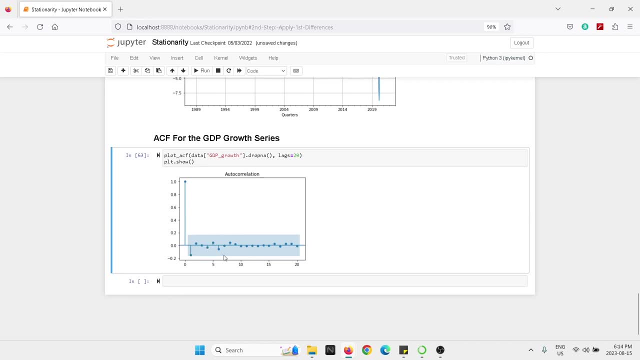 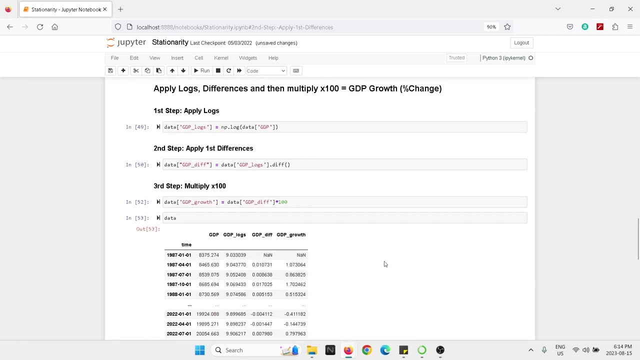 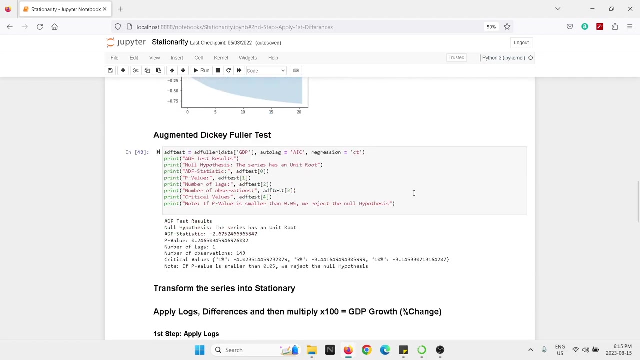 whereas now the decay is immediate. Also, as I mentioned before, remember the graph. This graph is wiggling consistently around a mean of zero and this one has a positive upward trend. So those are the differences between a non-stationary series and a stationary series. 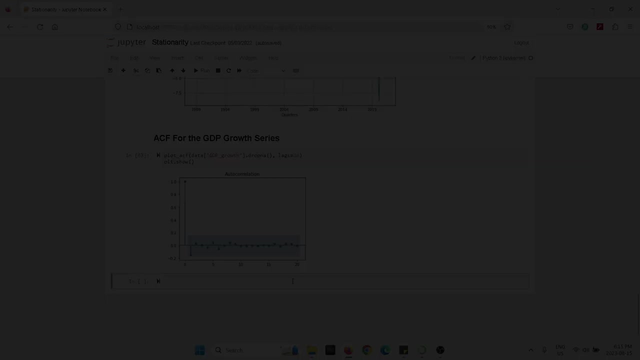 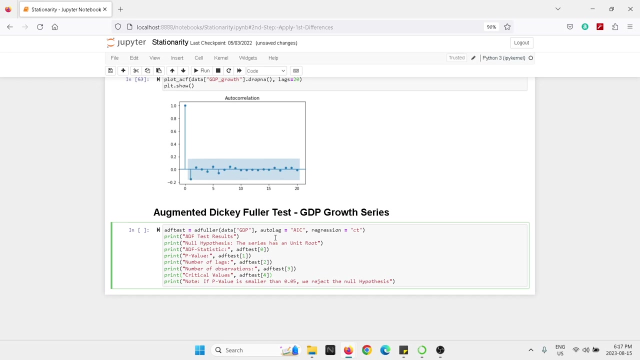 And now we can conclude with the augmented Dickey-Filler test. Let's now produce the augmented Dickey-Filler test on the GDP growth series. I have copy-pasted the code so we can save some time. Make sure that you modify this. 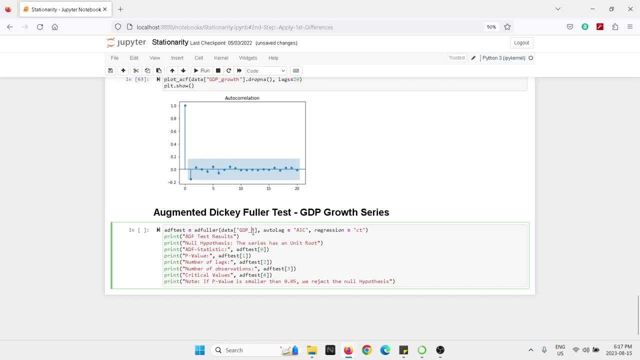 because we're not doing the test on the GDP series. Now it's on the GDP growth series And we need to modify the following. Remember that in this regression we had included a trend and a constant, But now, as you can see in this graph, 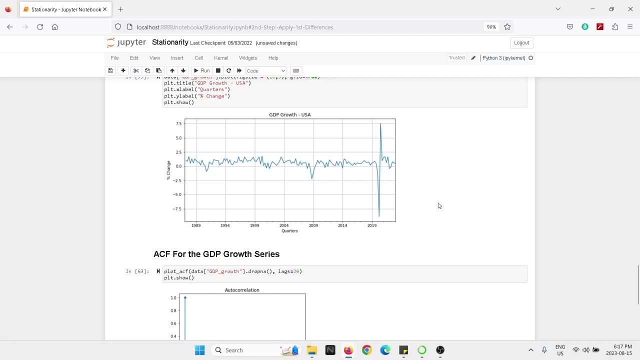 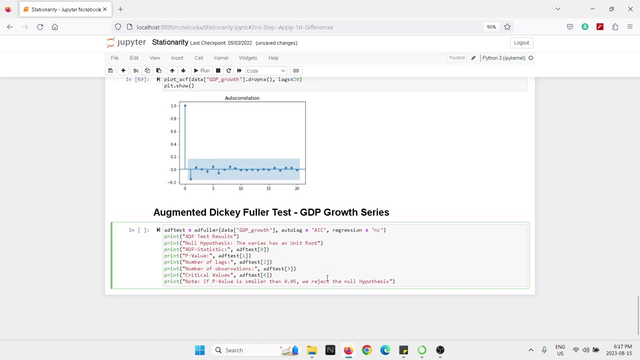 we don't have a trend and we don't have a constant. As you can see, there's no trend in here. So we're going to modify this and we're going to put NC, which is for non-constant or trend. 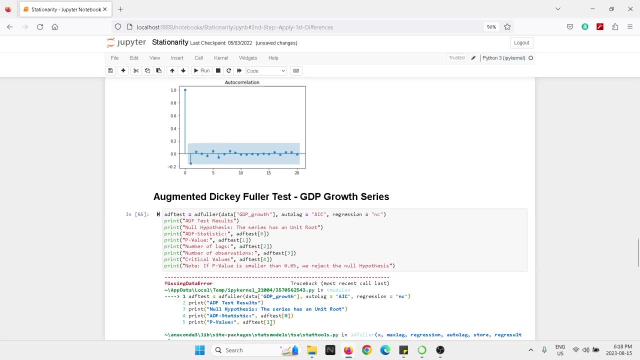 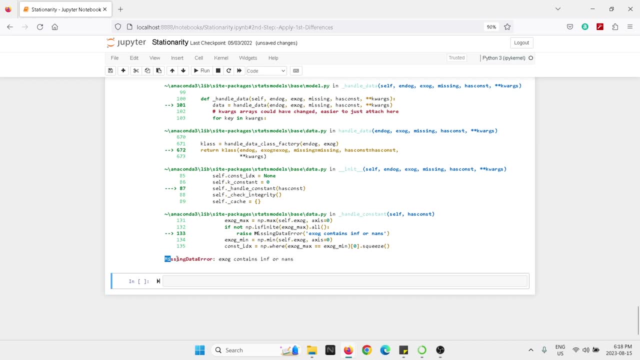 And we're going to hit on Run and see what we get. All right, so we're getting an error. Let's scroll all the way down. There's a lot of information in here, but it says missing data error, Exogenous contains inf or non. 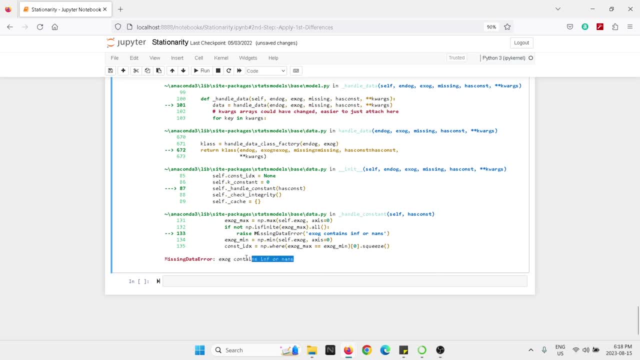 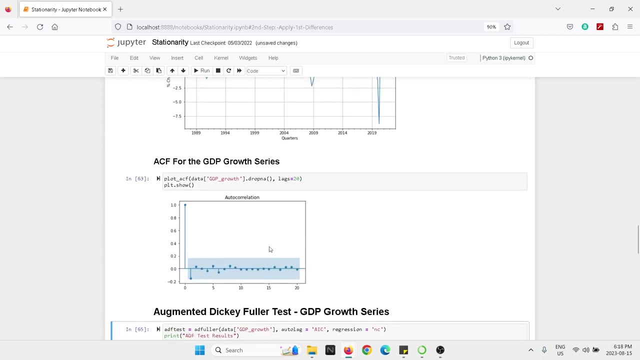 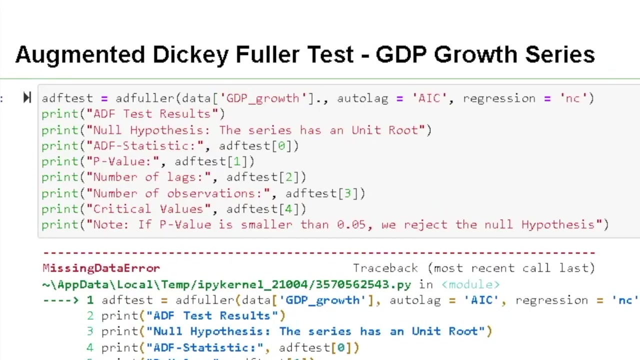 So it's basically suggesting that we have again. we are working with a series that has only rows with non-valid information, But we already know how to fix this error, because I already taught you how to do this in this case. So remember, we're going to go into here data and in this series. 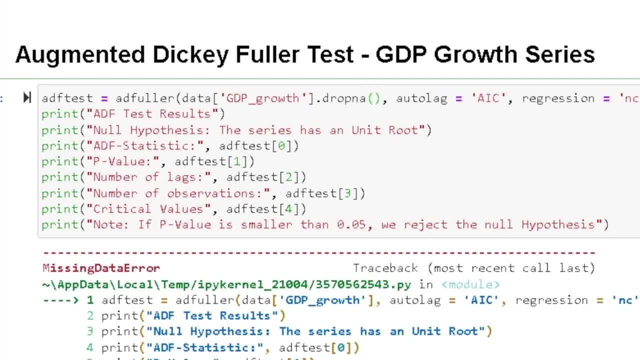 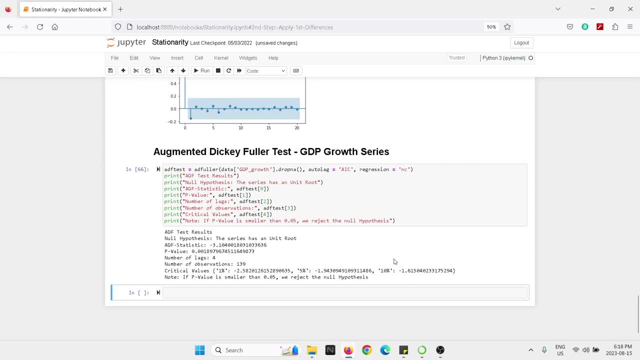 we're going to make sure that we drop those empty observations And we're going to run again and see if we get the error. And we don't get any error, So that's great. So we're getting the test results and let's take a look at the. 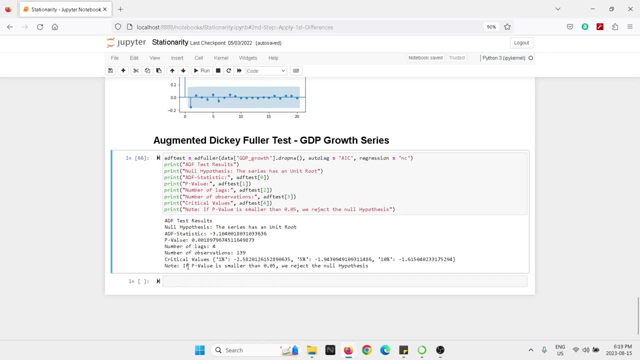 p-value. Remember, we wrote a note in here which says: if the p-value is smaller than 0.05, we reject the null hypothesis. And let's write something as well here. So if p-value is smaller than 0.05, we reject the null hypothesis. 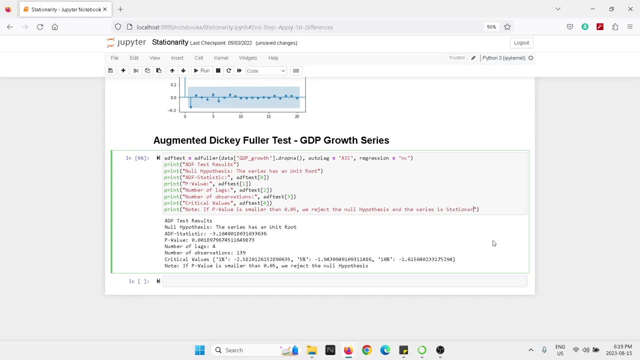 And the series is stationary. That's easier. So now we understand better. If the p-value is smaller than 0.05, we reject the null hypothesis and the series is stationary. OK, so the p-value is smaller than 0.05.. 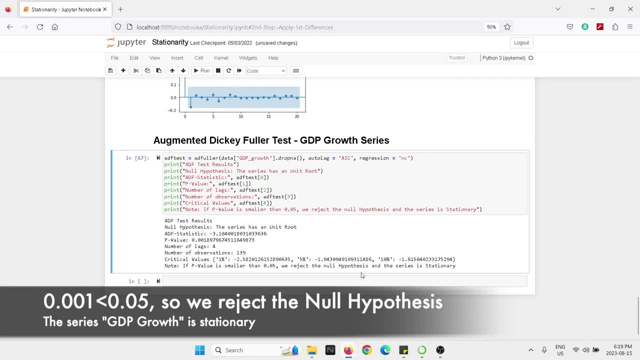 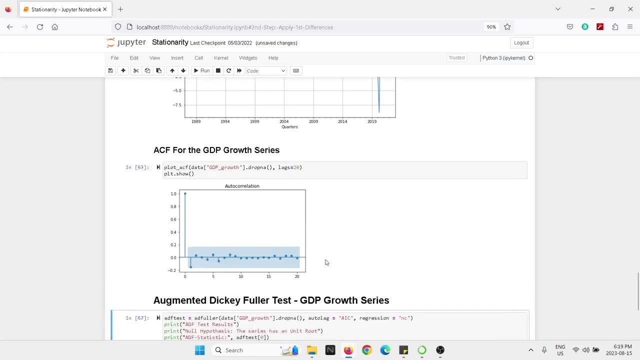 You can see 0,, 0,, 1.. So our series is stationary. We look at the graph: The series is detrending. We have that. the autocorrelation is suggesting that there is an immediate decay in the lags, So that's perfect. 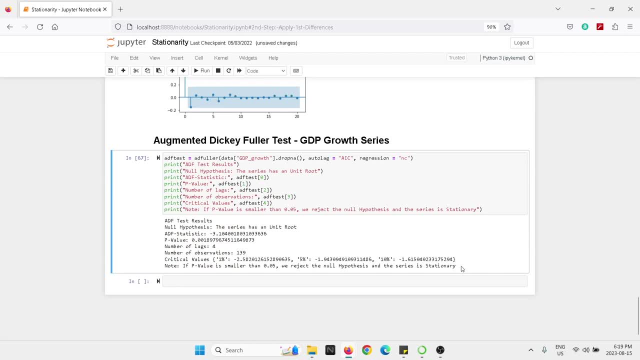 And with the augmented decay filler test we were able to determine as well that now my transformed series is stationary. This is going to be all the content for today. I would like to invite you to download for free the data set and the Python file. 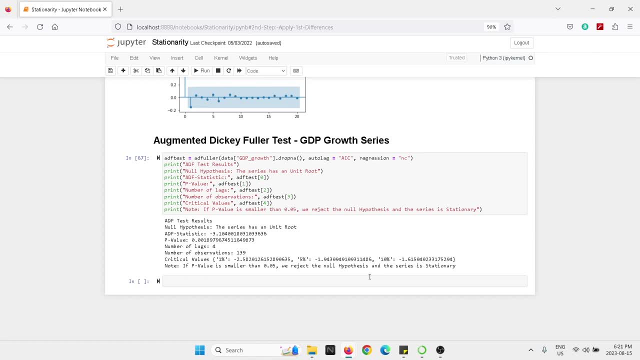 as well as a PDF where I have explained in very detailed way all the codes that we have used and what each line of code means, So then you can understand and try to replicate all this content. I would like to invite you to subscribe to my channel, because I'm going to be submitting more tutorials about time. 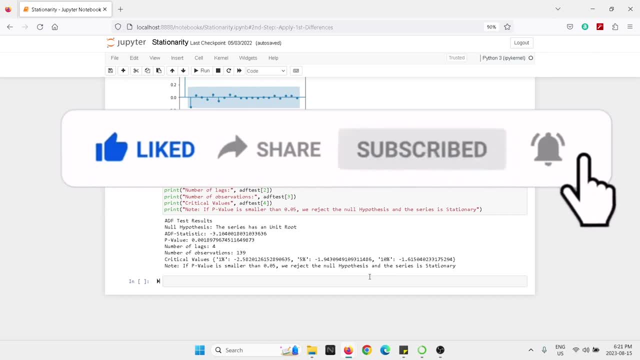 series analysis using Python. Next tutorial, I'm going to show you how to forecast GDP growth into the following ten quarters. we're going to be using an autoregressive model and I'm going to be explaining to you a little bit more. what are our regressive models, how we can. 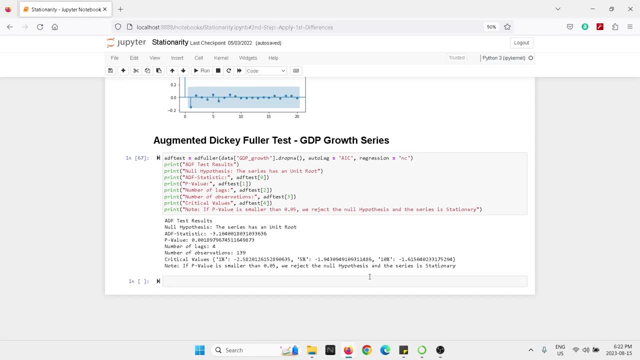 estimate them and then you will be able to see how we produce the GDP forecast. Please feel free also to share the content with anyone that you think that may find these tutorials interesting, And I hope to see you in the next video. Thank you very much. Take care. 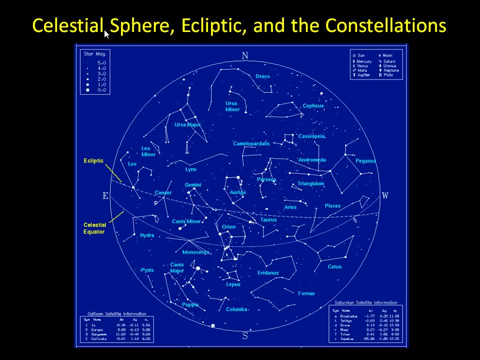 Hi class. this is a short video on the celestial sphere, the ecliptic and the constellations. This is material that's contained in chapter two of our textbook, and this is a pretty quick treatment of it. It's not comprehensive, so make sure to read this chapter, at least once. It tends.